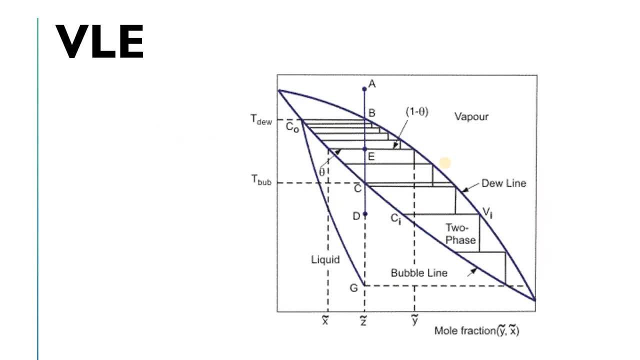 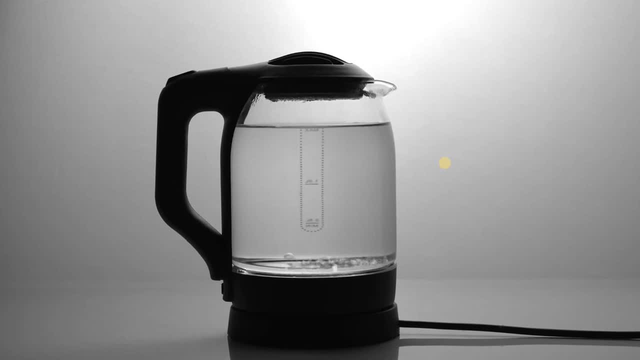 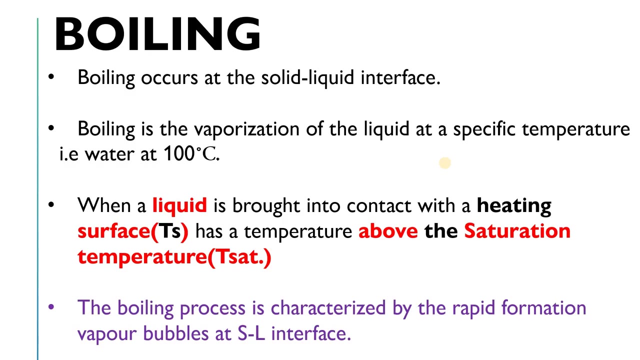 very, very interesting. i hope you will enjoy this video right? so if you are new in our youtube channel, please subscribe our youtube channel. press the bell icon so that you could get the latest notification. so let's start the video with what is boiling. so in our previous video, we 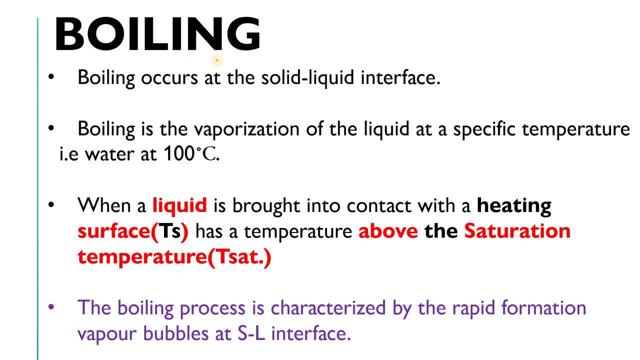 discussed about the evaporation and boiling. right, and we will also discuss about the evaporation, about the. what is the difference between the evaporation and boiling? right now, we will discuss first of all what is boiling, then we will discuss about the what is condensation, and after that we 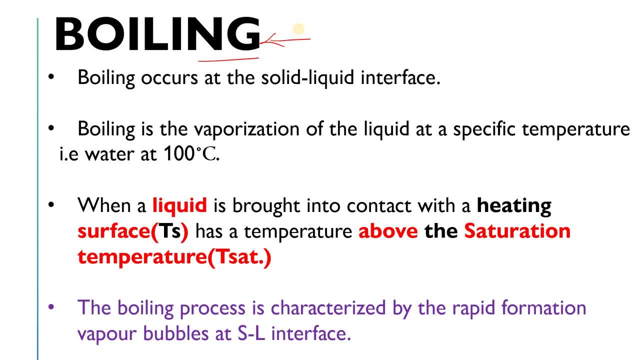 will try to understand that. what is the difference between them? okay, so first of all, we must understand that boiling occurs at the solid liquid interface, means in the case of the evaporation, it is the solid liquid interface. why? because, in the case of the evaporation, your liquid okay or you can. 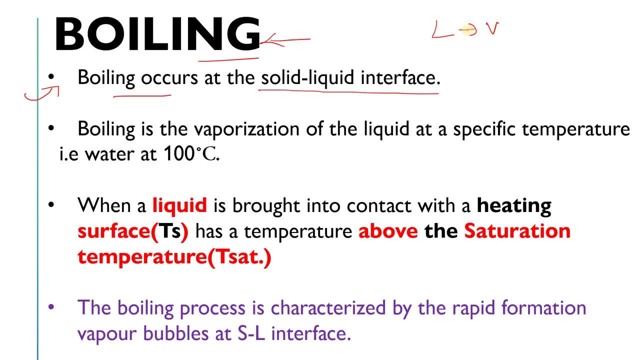 say simply, the phase of liquid changes into the vapor phase. right, in our case, there will be solid liquid interface. okay, we will understand that also. okay, let's suppose this is your one vessel, right, and there is the liquid. are you getting my point? now, what you are doing? you are heating. 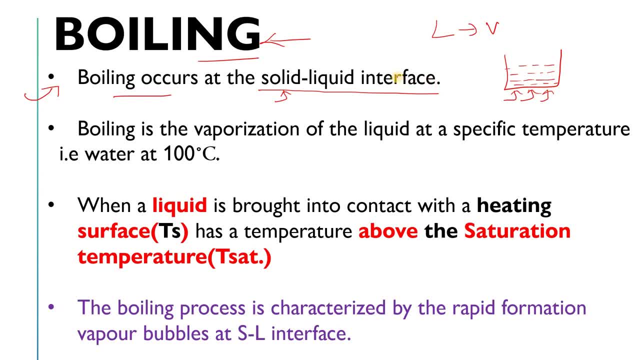 the surface. that surface is a solid right and this is your liquid. let's suppose the water right now. what is the meaning of the solid liquid interface? we are going to understand that in our next slide when we will see the what is boiling right now. you must understand that one thing as well: the boiling occurs at the solid liquid. 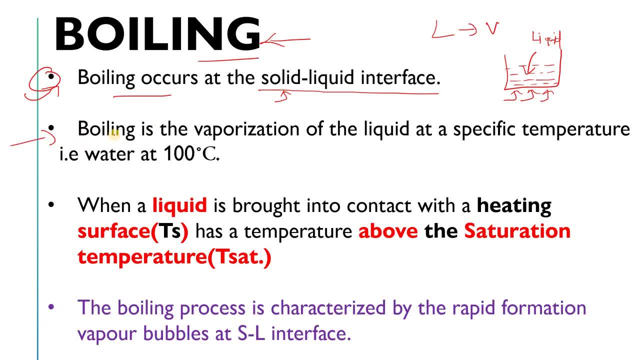 interface. okay. and what is boiling? okay, we have understood that. okay, boiling occurs at the solid liquid interface. now, what is the boiling? right, the next slide. we are going to understand that. Next question is that: what is boiling? So, actually boiling is the vaporization. 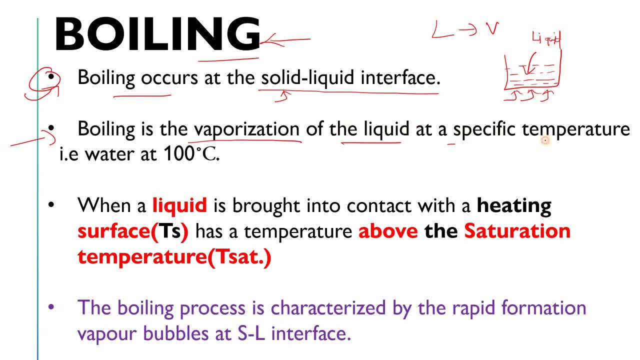 Boiling is the vaporization of the liquid at a specific temperature. OK, let's suppose, if we take the example of the water, So water boils at 100 degrees Celsius, when at one ATM means your atmospheric pressure is constant. Let's suppose so at one ATM, your water will be boiled at 100 degrees Celsius. 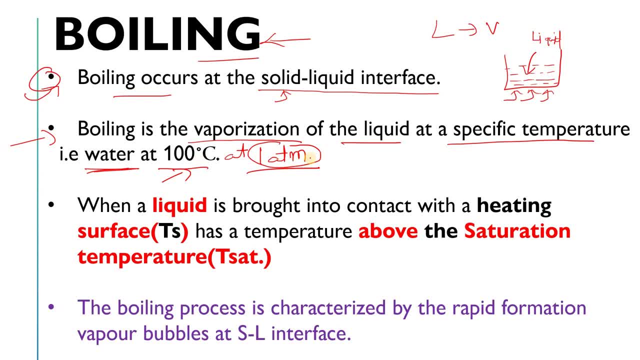 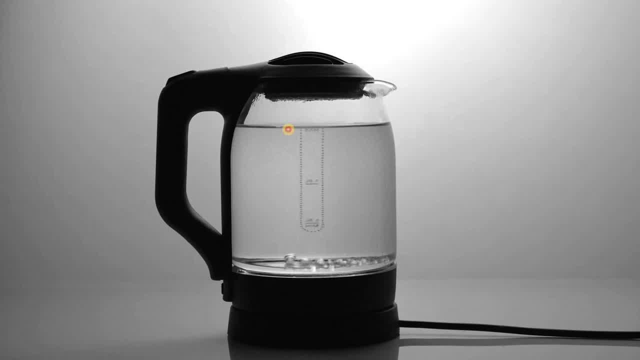 Right, So we will also understand that what will happen if we increase or decrease this pressure? OK, right, We have understood that. what is the boiling? Now let's see this example. OK, so what is happening here? Initially, the bubbles are forming at the surface, at the solid surface. 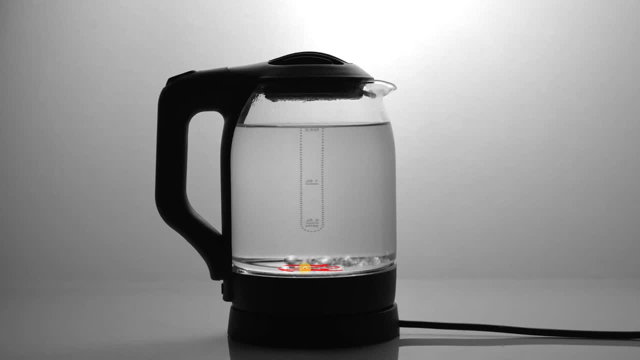 Right, But we know that in the case of Of the boiling, you will see that your bubbles will be here. So what is happening here? as you are increasing the temperature, so your rapid formation of the bubbles are increasing means your bubble formation are increasing and you can see here the bubbles are forming here. 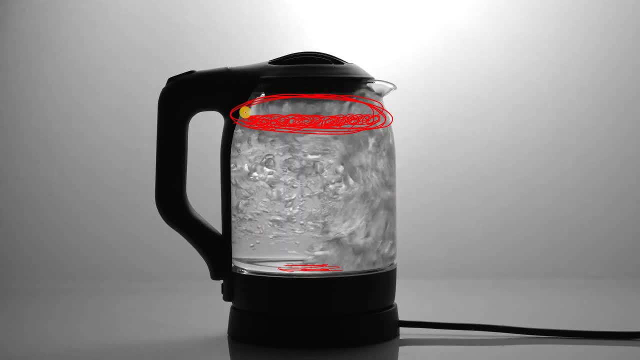 OK, the bubble formations are there. Right, This is the boiling. OK, this is the boiling. Please do not confuse this with the evaporation. OK, You can also see our previous video where we discussed about the evaporation and boiling. 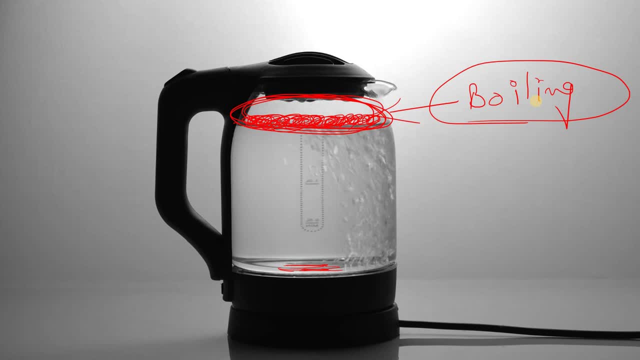 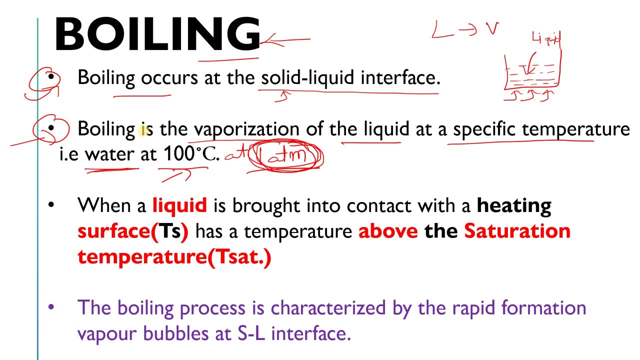 OK, So this is the mainly the boiling. OK, Now just see, here we have understood about the what is boiling? OK, In the case of the boiling, the bubbles will be. you can, visually, you can see the bubbles. OK, At this surface you can see the bubbles, but starting it comes from. OK, start it starts from here. 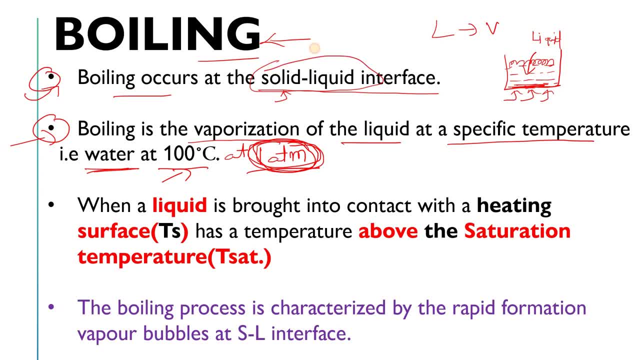 That's why I have written here: solid liquid interface. Please try to understand it, because I am trying to explain you the concept in a layman language. OK, Now we know that. what is boiling? right, when the boiling will be occur? OK, What is the condition? 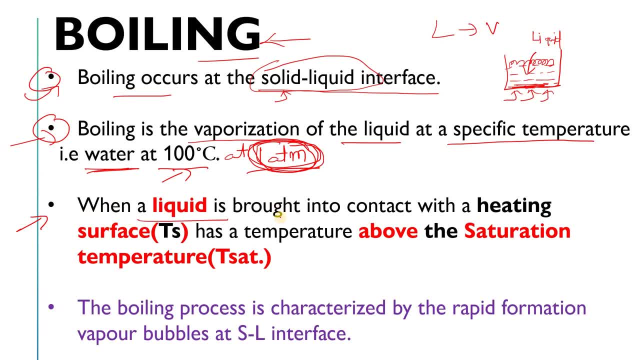 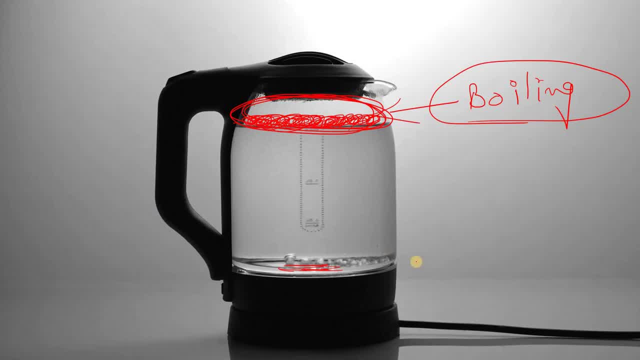 So the boiling will be occur when a liquid is brought in contact with a heating surface. OK, In our case there is the coil. This is your coil. OK, You can see here. OK, This coil will be Connected with the electrical supply we are giving here. 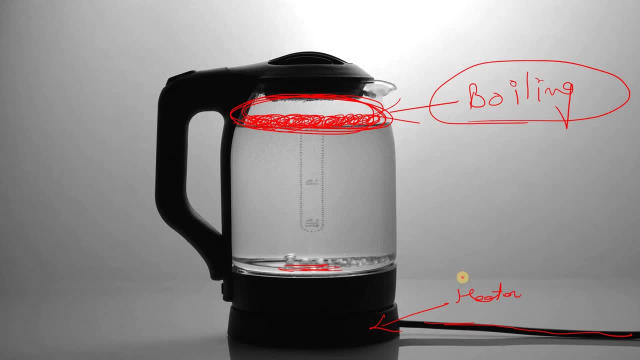 This will be your heater. OK, And coil, we can say simply electrical heater. It will be your electrical heater. Now what will happen? that it will heat the surface, So, OK, it will heat the surface. So there will be one plate. 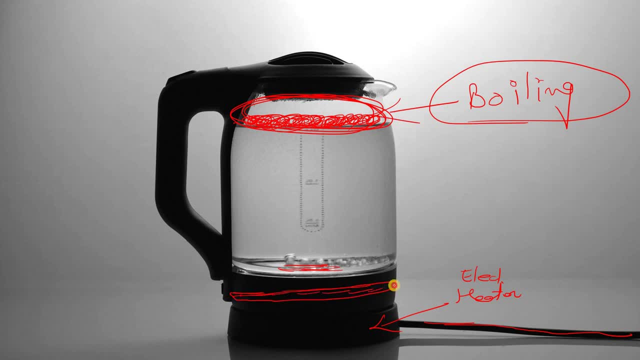 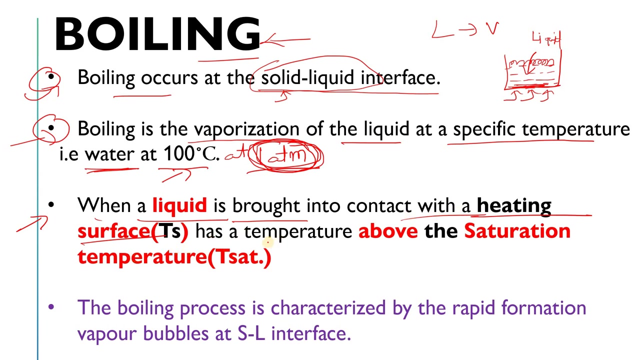 OK, That plate will be becomes hotter as you will increase, like as you will give the supply. So it means what happens here: This metal surface of this solid surface or heating surface, temperature increases. Let's suppose it's temperature is TS, Right? So what you are saying? you are saying that when a liquid is brought in contact with our heating surface has a temperature above the saturation temperature- saturation temperature of a liquid at that pressure. 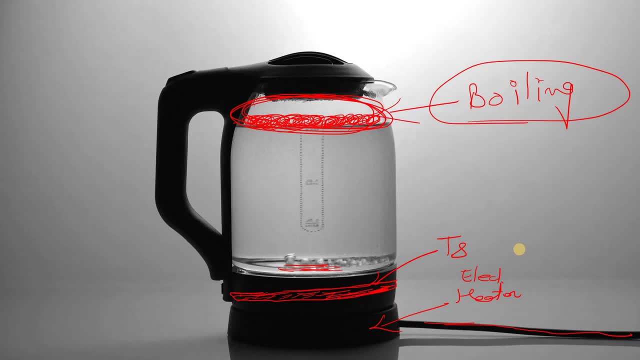 This point is very, very important. OK, Now see, in our case, This heating surface will have some temperature. OK, Now, what am I saying that? I am saying that this liquid, OK, There is the water, Right, So let's suppose this water. 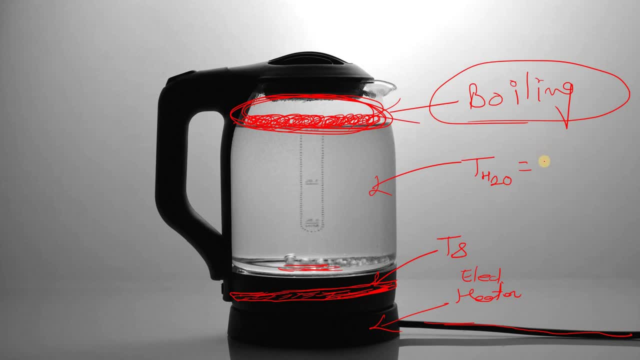 I'm writing here the temperature of the water right now. Let's assume that its temperature is 110 degrees Celsius. OK, And it is at the room. temperature means it is at the room, So it will be. the pressure will be one atmospheric pressure. 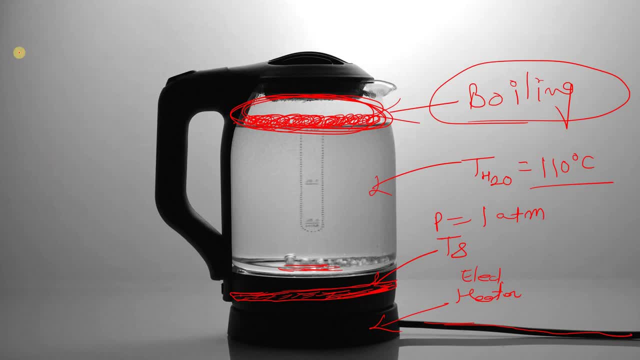 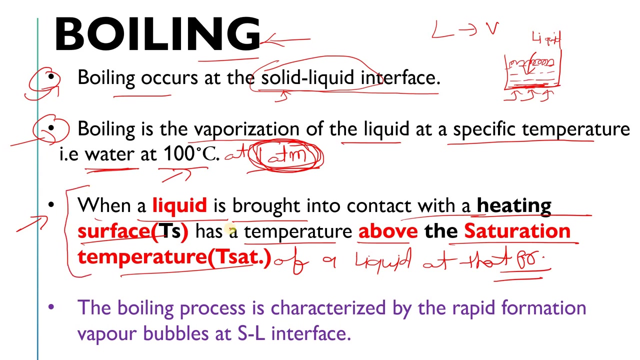 Right, So now we know that at one atmospheric pressure, at one atmospheric pressure, that saturation temperature of the water is 100 degrees Celsius. Right, So now, what will happen? The boiling will occur. Now, what will happen here? The boiling will be as if you, if you read this statement right? 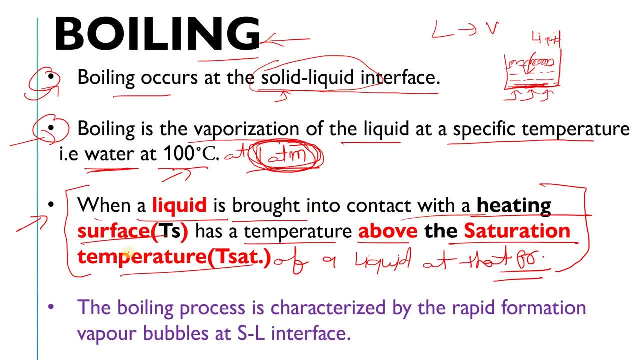 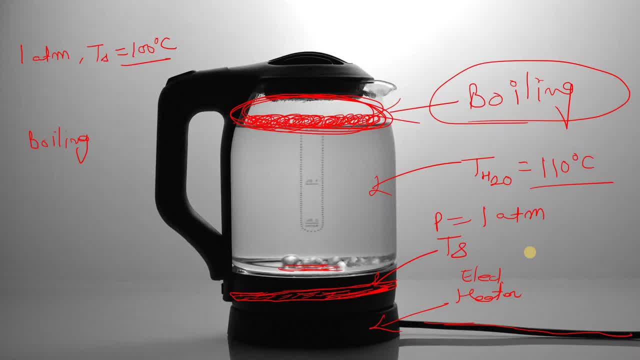 When a liquid is brought in contact. contact with a heating surface has a temperature above the saturation temperature of a liquid at that pressure. so see here now what will happen: that your boiling will be occur. are you getting my point? what i want to say? this is the very, very simple right now means your liquid temperature is. 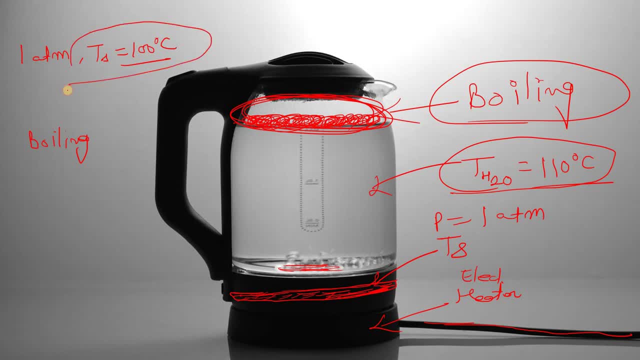 above the saturation temperature of a liquid or a water. okay, means your saturation temperature is going to be constant at a particular pressure or particular pressure and temperature. are you getting my point? so this is the. this is. this is about the boiling right. okay, this is very, very. 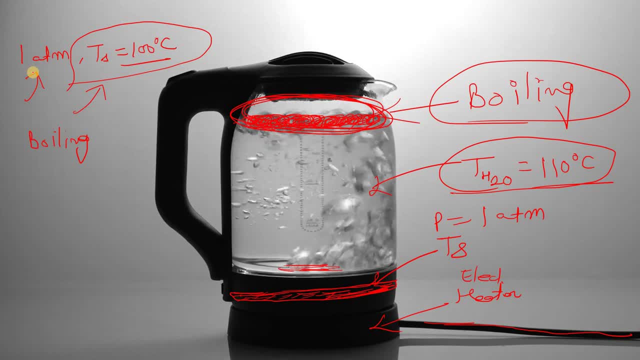 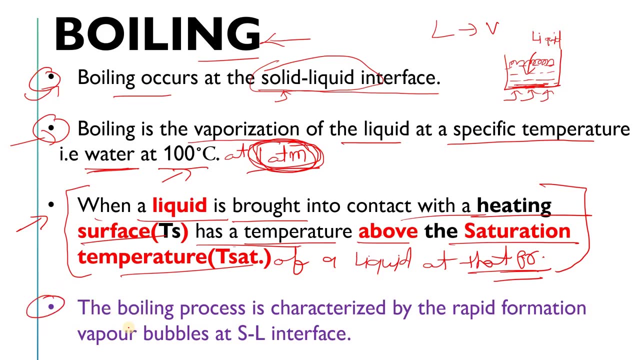 simple now. if you have any doubt till now, please let me in the comments box so that i could explain you in a better way, right? so that's why i have written here that, okay, the boiling process is categorized means what type of the boiling is. that means pool boiling. 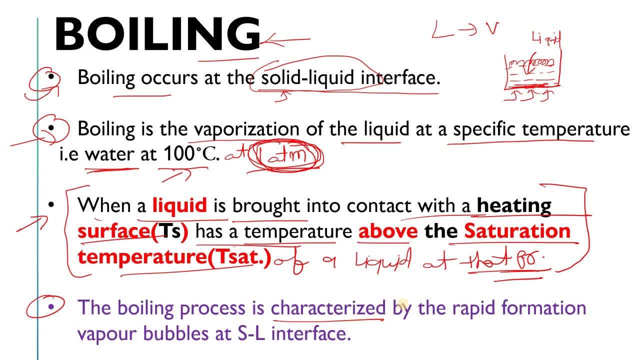 sub cool boiling, film boiling or natural boiling. so there are so many types of the boiling we will. we will also study that. okay, like the boiling categorization or types of the boiling we will also discuss in our next video, right? so boiling process is categorized by the rapid formation of 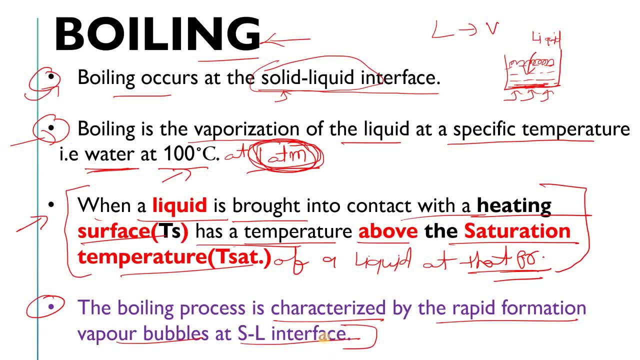 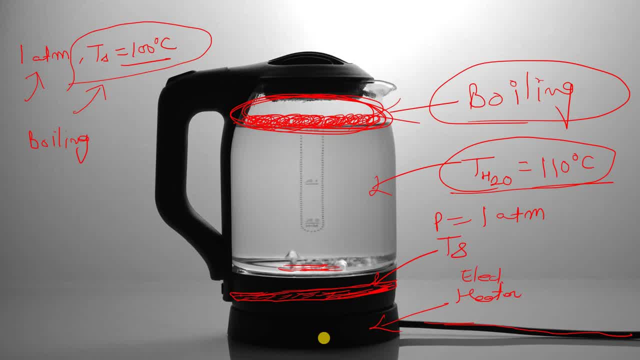 the vapor bubbles at solid liquid interface means, as you will increase the temperature, so what will happen? that the rapid formation of the bubbles will also increase. right, so that we are saying that it depends upon the temperature as well as your excess temperature means it depends upon the, it depends upon your delta t. okay, that is. we simply say this is the excess. 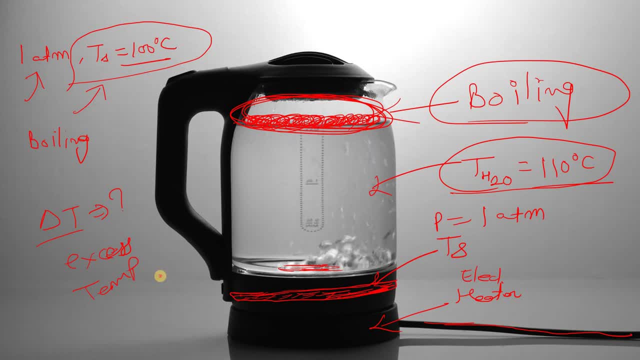 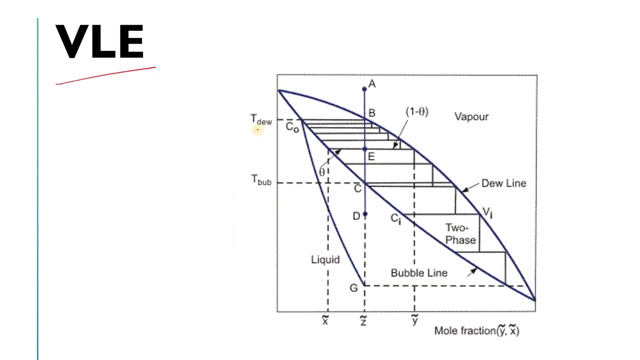 temperature. okay, so we will discuss about it in our boiling curve video. are you getting my point? so this is all about the boiling? okay. so here, if you will see that this is your vapor liquid equilibrium curve, okay, which is plotted or plotted between the temperature versus your mole fraction. 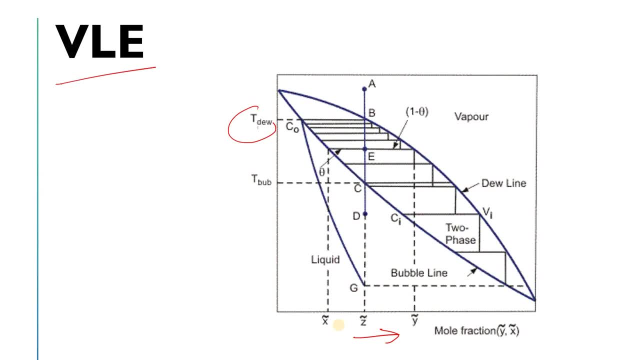 okay, let me in the comments box that: what is the mole fraction? so mainly in this case, this is the binary solution. okay, let's suppose there will be only two component, a plus b, right? so i am not going to detail of the vapor liquid equilibrium, i am just simply. i am just trying to explain you that. 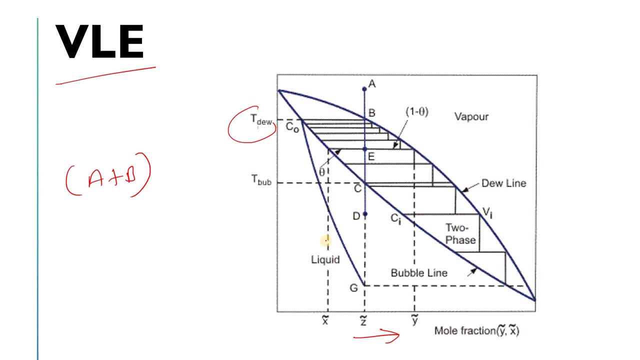 what is the boiling? okay, so you will see that the vapor liquid equilibrium is a very important component of the liquid equilibrium curve. okay, so you will see that if we this is your liquid region, this one is your own, this one is your complete liquid region and this will be your vapor region. 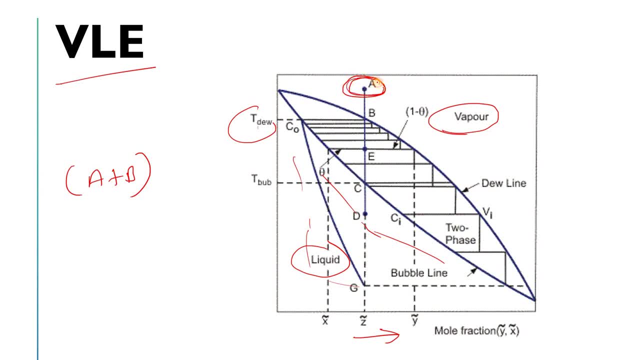 okay, now, let's suppose at this point what will be here here will be vapor, simply okay, and same as what will be at g: there will be liquid. are you getting my point? what i want to say? okay, so now, what you have done, there was your liquid. okay, your liquid was here. okay, at that point. 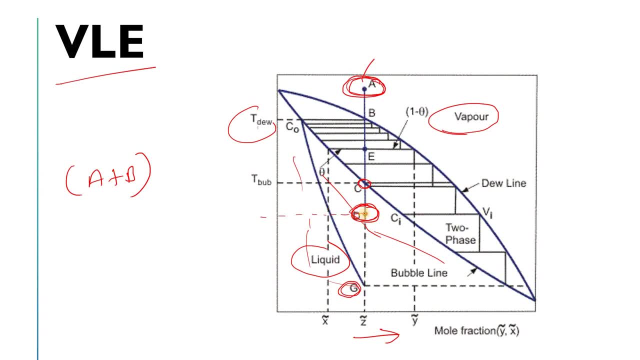 your liquid was here, okay. now if you increase the temperature? so okay. so what will happen? that after some time your temperature will be increased. right, your temperature will be increased and let's suppose it reaches here. okay, and this is your bubble point. okay, so what will happen if you take? 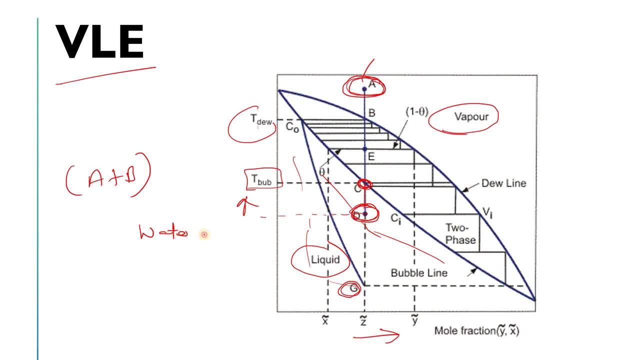 the example of the water. so your water will start boiling. okay, in that case, the boiling will start. this is your vapor liquid equilibrium curve. okay, so what will happen if you increase the temperature bubble point? okay, in the, in the case of the water, that is 100 degree celsius right now. if you further, 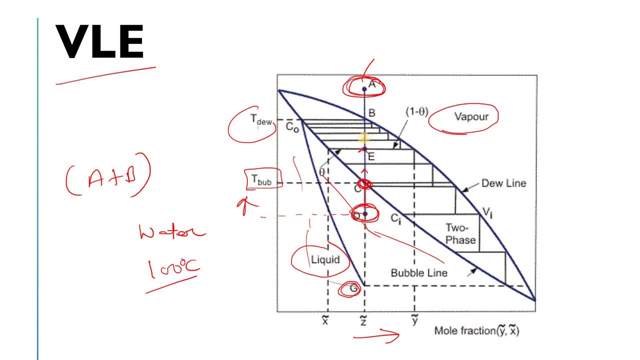 increase the temperature. so what will happen if you further increase the temperature so the water is not completely boiled? okay, there will be the liquid and you will see the boiling. okay, so means what will happen? that in this region there will be liquid plus vapor means boiling has started. 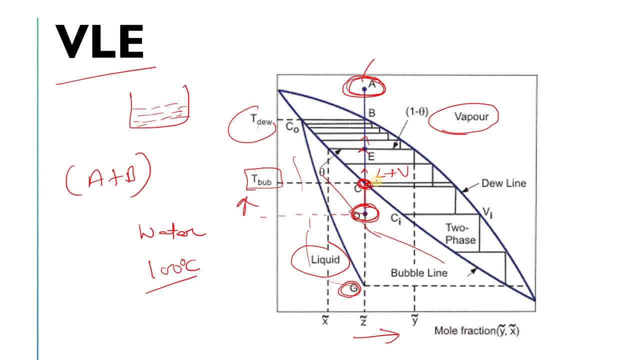 okay means vaporization has been started, but if you increase the temperature, so what will happen? it is not completed. so in this region means from c to b, there will be what. what will be here? there will be liquid plus vapor, but the boiling has started. okay till b. are you getting my point? 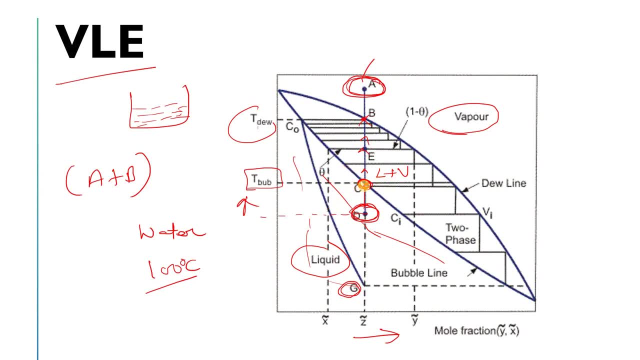 what i want to say: right, this is your boiling. okay, now, if you will, simply, if you simply keep your temperature constant, so what will happen? that only with this rate your boiling will be. this is your tie line, nothing else. are you getting my points? and this one is your bubble line, a bubble. 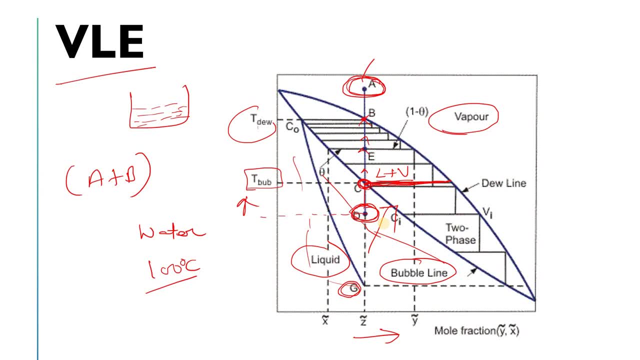 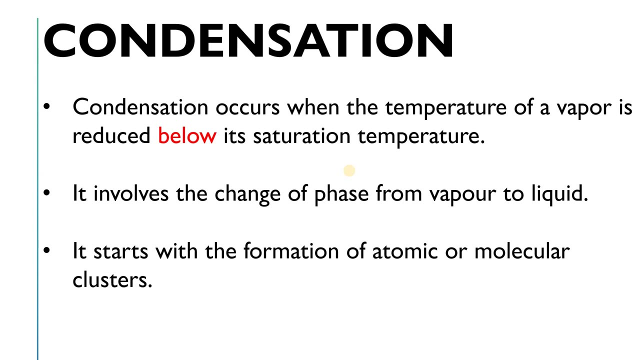 curve line. you can simply see. are you getting my point? this is very, very simple. this is your bubble point, or. t means bubble temperature. okay, from this, from this temperature, your liquid will be start boiling right now. let's understand that. what is condensation? okay, after that, we will also. 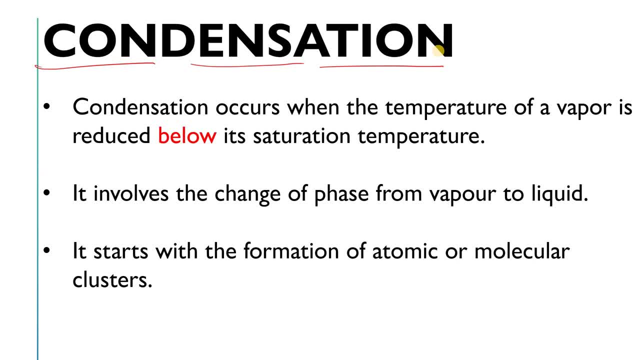 come back to this, which is condensation. okay, after that we will also come back to this, which is your vapor liquid curve. now, condensation occurs when the temperature of a vapor is reduced below its saturation temperature. we have already discussed about that. what is saturation temperature right now? first of all, understand that. what is condensation? actually, condensation is nothing but. 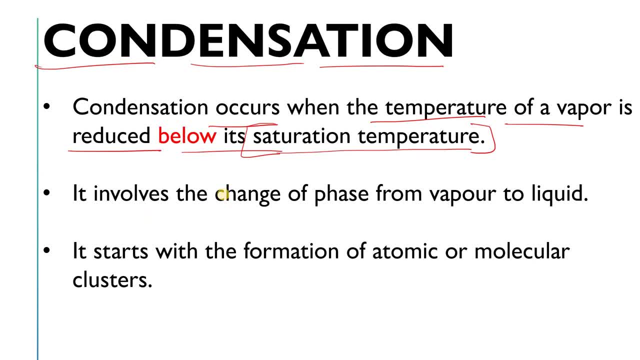 it is the process. okay, in the both means condensation, and in the boiling there will be the fluid motion. okay means it is a convective heat transfer, right. so in condensation, okay and simply we can say: condensation involves the change of phase from vapor to liquid. okay, in our, in the 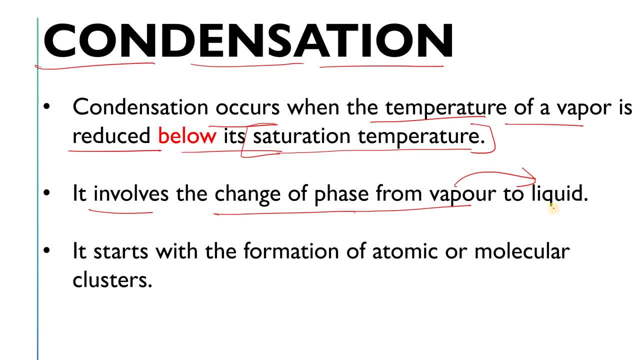 case of the leak. in the case of the evaporation, your liquid was converting into the vapor, okay. same in the case of the boiling: there was what? what was happening there? the liquid was vaporizing, okay. and in the case of the condensation, what will happen? that your vapor will be convert into the liquid. are you getting my points? so how it happens it. 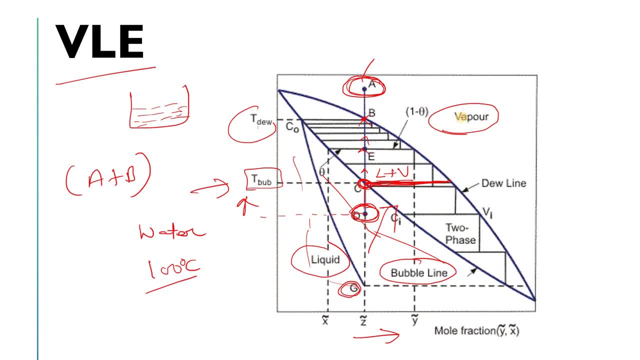 happens that let's suppose see here, now there is the, there is the vapors. let's support there, there is the vapors of the, your waters right now, what you are doing here, and let's suppose you are at a right now what you are doing, you are simply reducing the temperature. okay, so, as you will, 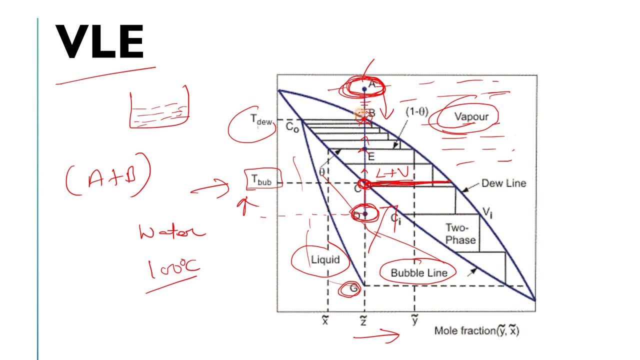 reduce the temperature. what will happen? that at point b the one drop means first drop of the vapor. first drop of means your vapor will convert into the liquid, means first drop of the liquid will come or form. simply you can say okay at that point. okay, and that point is called the due point or due. 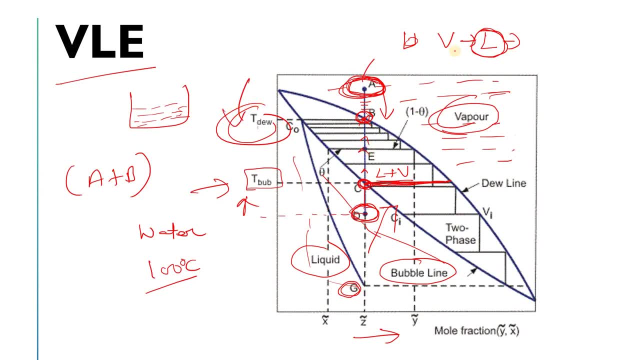 temperature. simply you can say a dew point. you can say: are you getting? my point means simply you can say: when you reduce the temperature of the vapor, okay, so at that point where the first drop of the liquid forms is called the dew point, okay, so this is your dew point. and if you will, 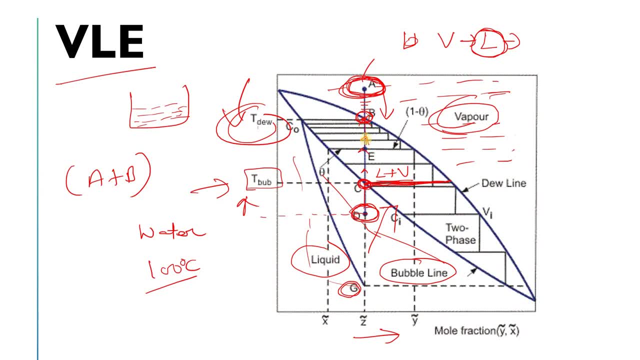 further reduce the temperature. so your web means your condensation will be occur. so from here, the condensation has been started right and that's why this is your dew line. this is also very, very important when you are studying the condensation, right. so, dew point, dew line, these, these topics. 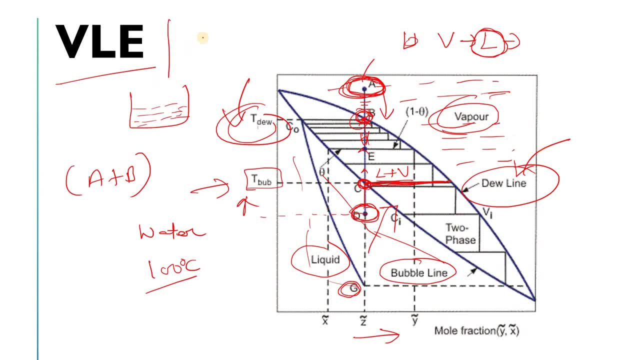 are very, very important. let's suppose if you are an engineering student or engineer, so you will have seen that in industry there are cooling tower right. so in the cooling tower the dew point plays a very, very important role. are you getting my points now? in this region, the boiling and 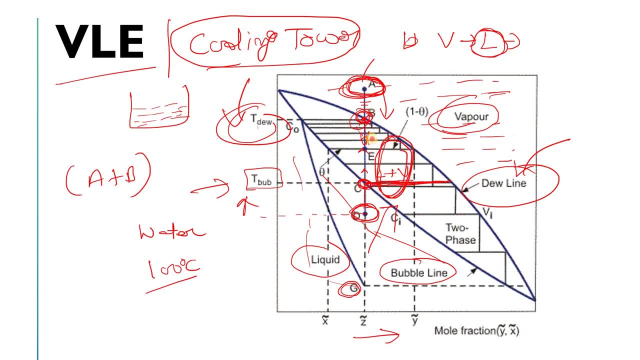 condensation both occurs right. in our case, what we are doing, we are simply reducing the temperature. so your vaporize like your condensation is occurring, okay, and in our, in the case of the evaporation, we will have seen that if it is a closed container, okay, and we are heating it. so what happens here? the vaporizes like evaporation. 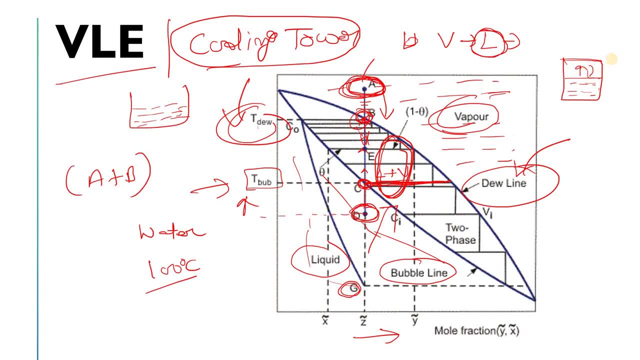 occurs as well, as condensation also occurs. okay, we discussed about it in our evaporation video. are you getting my point, what i want to say? so that is the very, very important. you must understand that. you have to understand that. you have to understand that. you have to understand. 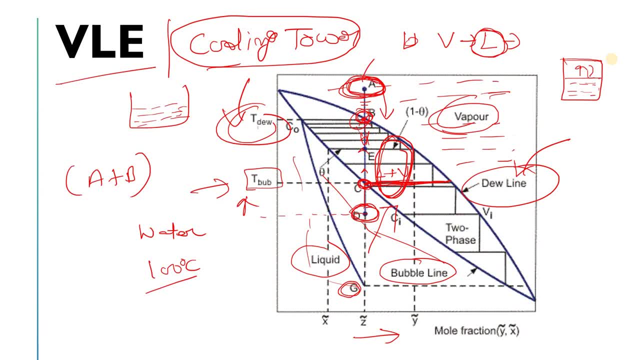 that point as well. so when the condensation will occur? simply when you will reduce the temperature. okay, so in our case, what was the saturation temperature? so saturation temperature of water is 100 degree celsius. simply what you have to do for the condensation: you will have to reduce the. 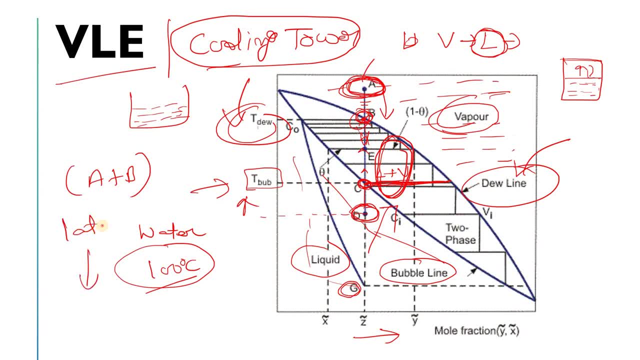 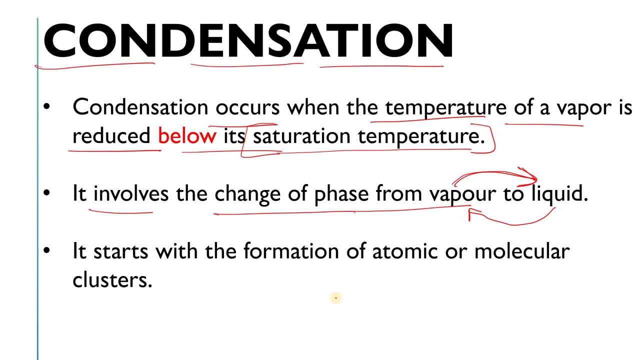 temperature below the 100 degree celsius at 180 m. okay, again and again, i am like focusing- or on the temperature and pressure. okay, because these two terms are the temperature and pressure. okay, because these two terms are the temperature and pressure. okay, because these two terms are the temperature and. 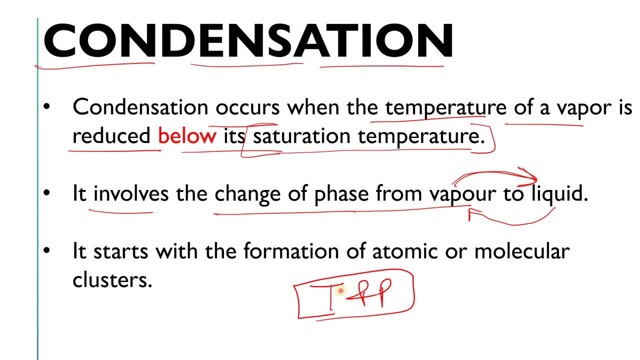 pressures are very, very important in the case of the condensation and the boiling. right, you will have seen that, like, if you go in a high altitude, your pressure decreases. right, so you will have. you will have seen that in that case the boiling also alter, right so as the temperature, as the pressure. 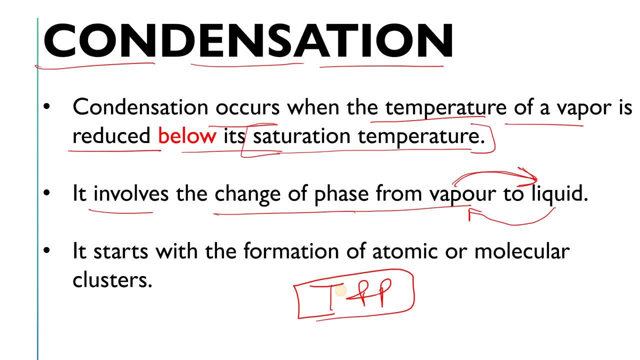 will like reduce or increase, right? so your boiling temperature will also reduce or increase because the temperature is simply, you can say, directly proportional to the pressure, right? your temperature is directly proportional to temperature. so can you let me in the comments box that why in the hill station your liquid boils at lower temperature? very, very simple. please let me in the comments box. 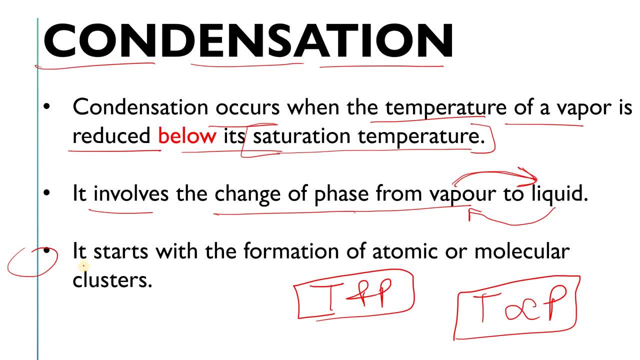 right now. in the last what i have written, i have written that condensation starts with the formation of the atomic or molecular clusters. okay, this is nothing but like. let's suppose if there are so many vapors and they comes together, so what will happen? that it will make one. 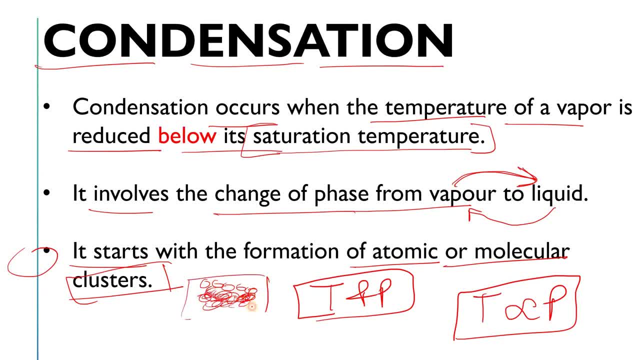 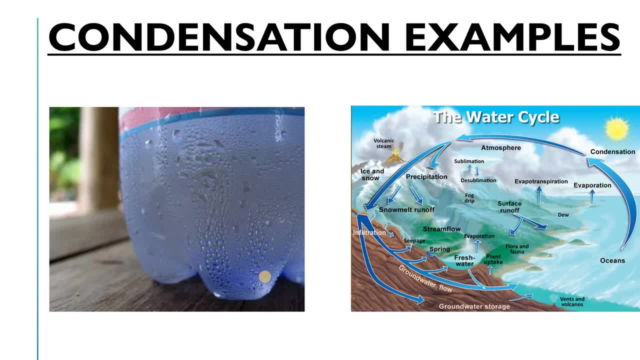 droplets you can see, or the cluster you can see, and this is, and after that it becomes the one droplet of the liquid, and this is called the condensation. okay, now simply see here there are the two examples, and both examples are the daily life examples. 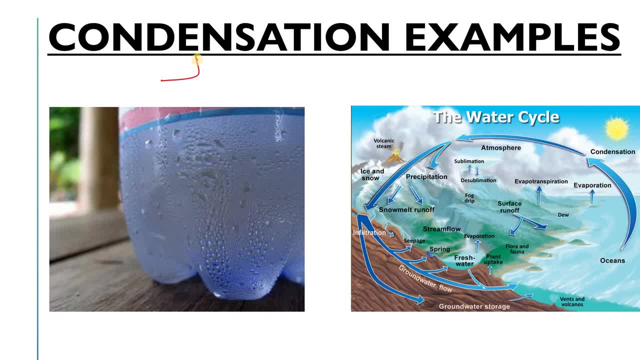 or the journal examples of the condensation right, i'm not going in an industrial one. this bottle was in a fridge refrigerator. now, simply what you have done: you just keep this bottle at the room temperature or at the table. so what will happen? that the water vapor in the air will come in contact with this bottle, because this 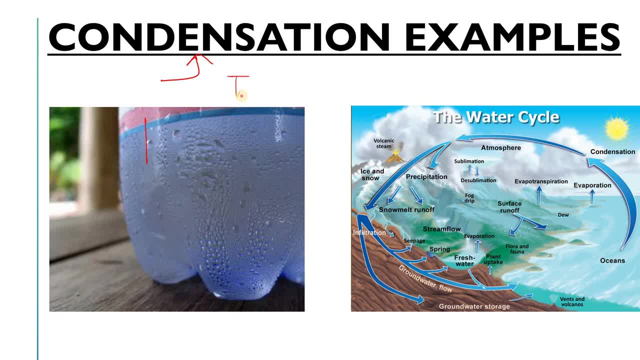 temperature. okay, this bottle has a some temperature. that is the cooler, that is cold, or i'm simply saying that less than the your atmospheric temperature. okay, the room temperature. so what will happen? that that vapor will convert into the liquid. okay, because, simply, the temperature is below than the situation temperature. okay, so what will happen? you will see, there is the droplets of 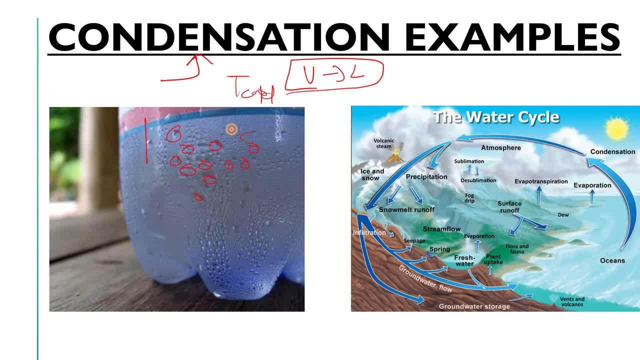 the liquid. okay, so how this vapors are converting into the liquid because of the cluster. okay, they are simply like coming together, okay, making the cluster or the- you can say the droplets, and you can simply see physically by the eyes, visual inspection, simply, you can do here, simply you. 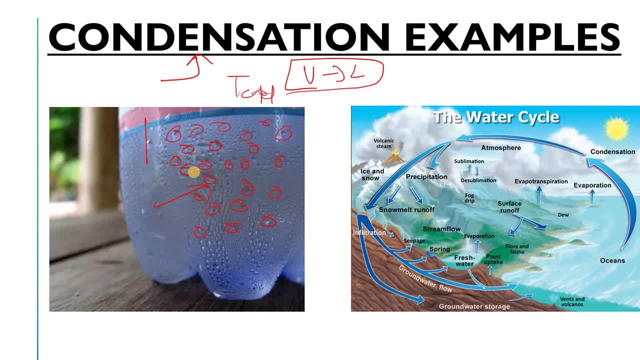 can do here and you can see these clusters. okay, this is the condensation, right? another example of the condensation is the water cycle, like in a sea or in the ocean. you will have seen that there is the evaporation occurs, right, okay, after the evaporation, the clouds forms. how these clouds forms? these clouds forms because of the condensation. 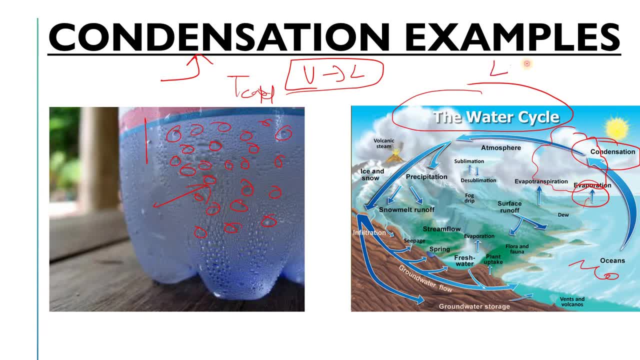 okay, evaporation means simply, your liquid converts into the vapors, right? but in the case of the condensation, it, your vapor, will convert into the liquid. are you getting my point, what i want to say, right? so these are the things that will happen after the evaporation, right after the evaporation. 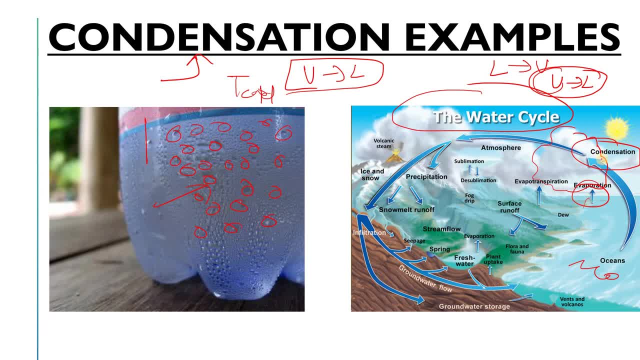 are these some examples of the condensation. can you explain this process? okay, this is very, very simple, because, because of the condensation, the clouds forms. now how the rain circles, rain comes. okay, very, very simple. okay, please let me in the comments box. are you getting my point now? okay, 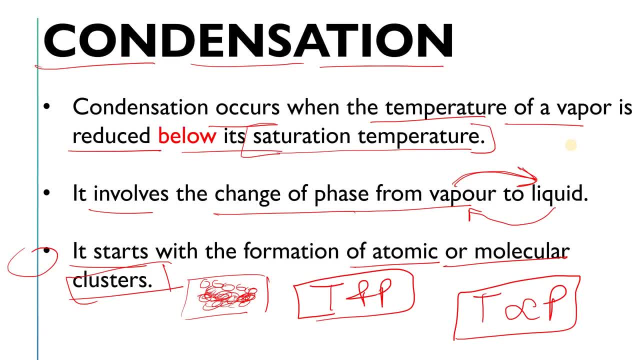 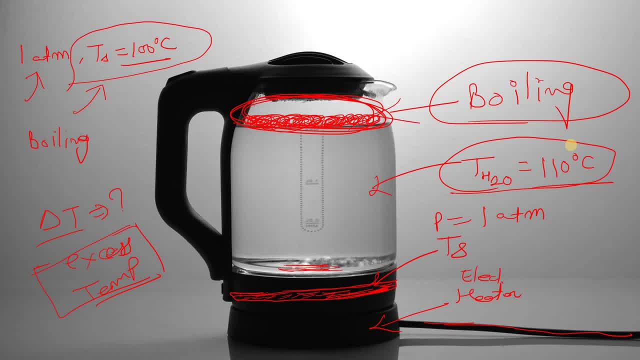 so these was the. so these was the difference between the condensation and the boiling. simply here we do not like distinguish between the condensation and the boiling, or simply here we do not like distinguish between the boiling and condensation. but if you want to know about it, like, what is the? 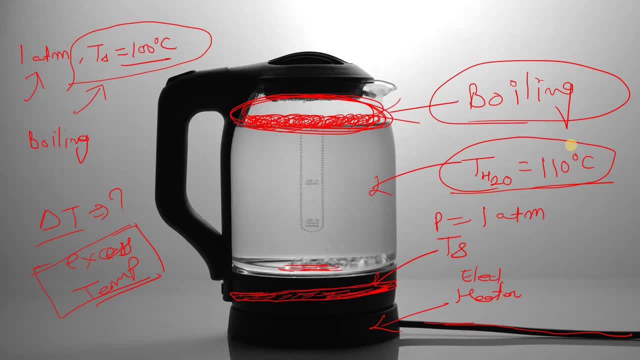 difference between the condensation and evap, like condensation and boiling, so i could simply tell you like, in the case of the boiling, if we like, if we discuss about the boiling, so boiling is the vaporization right of a liquid at a particular temperature. means you will see here the bubbles. 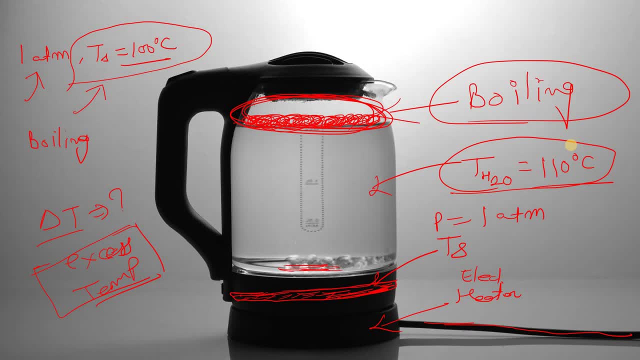 at the top surface. are you getting my point in the case of the water? so at 100 degree celsius your water starts boiling. at 100 degree celsius, your water starts boiling. at 100 degree celsius, your water starts boiling at a one atmospheric pressure. this is very, very important. 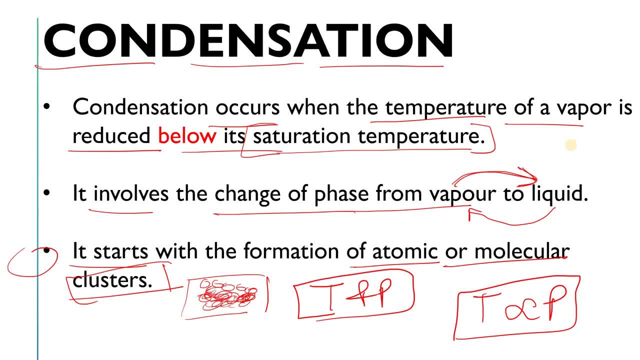 but in the case of the condensation, if you will see here, so condensation in the condensation, what happens? that your vapors converts into the liquid. and when you reduce the temperature, are you getting my point? this is also very, very easy. so your temperature should be below the saturation.